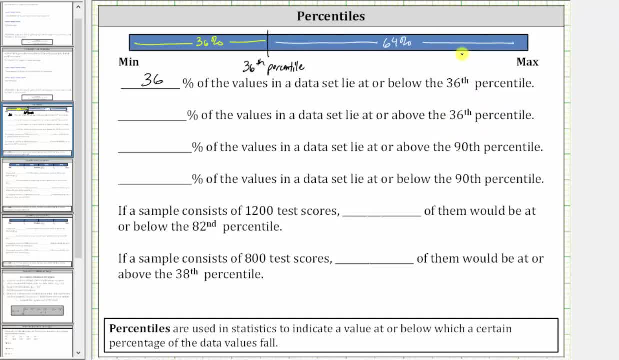 which is 66%. So 64% of the values. these values here on the right. The next two statements involve the 90th percentile. The 90th percentile would be approximately here where now 90% of the data values are at or below. 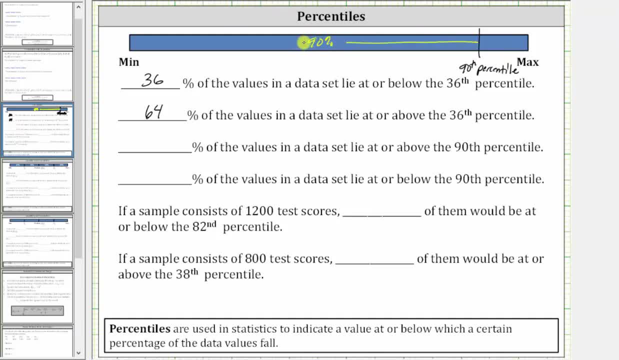 the 90th percentile, which are these values here on the left? and therefore, 10% of the data values must be at or above the 90th percentile, which are these values here on the right. So reading carefully. the next statement asks: 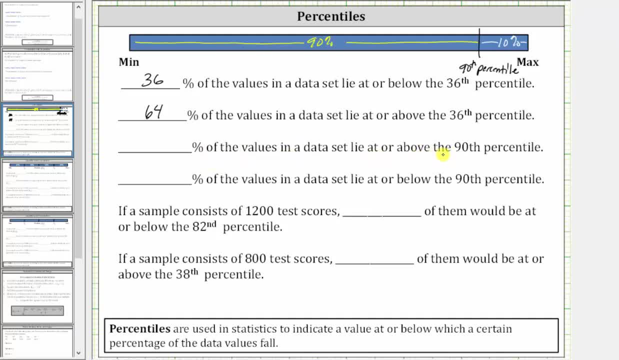 for the percent of values in the data set that lie at or above the 90th percentile, which is 10%. the values on the right. Next, we want the percent of values in the data set that lie at or below the 90th percentile, which is 90%. 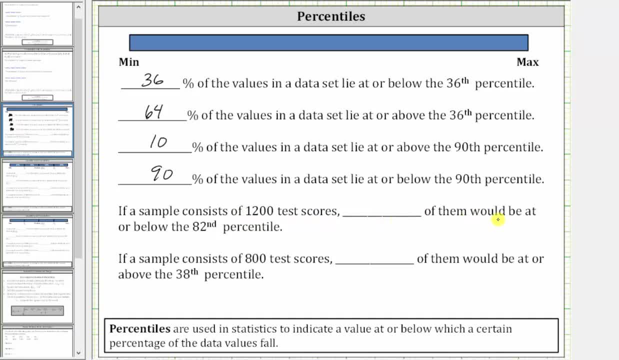 Next, if a sample consists of 1,200 test scores, how many of them would be at or below the 82nd percentile? Because we want the percent of test scores below the 82nd percentile, this is going to be 82% of 1,200. 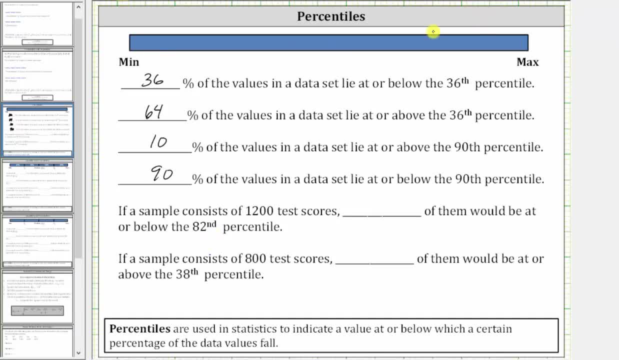 But just to show it on the graph: above the 82nd percentile would be approximately here, where 82% of the data values are added below the 82nd percentile, which means 100% minus 82% or 18% of the data values. 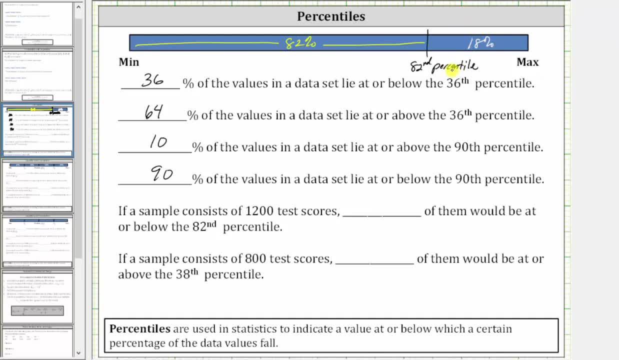 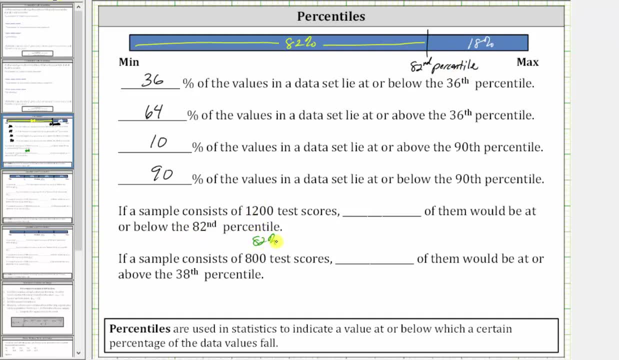 must be at or above the 82nd percentile. But again we're looking for the number of test scores below the 82nd percentile, which is 82% of 1,200.. To find the percent of a number, we convert the percent to a decimal and multiply. 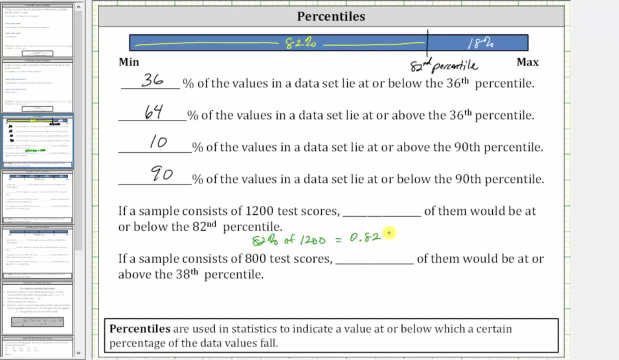 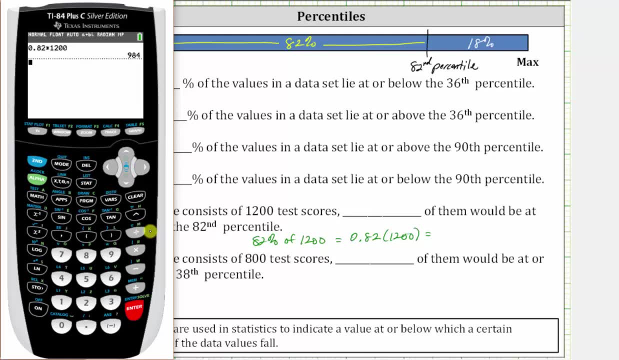 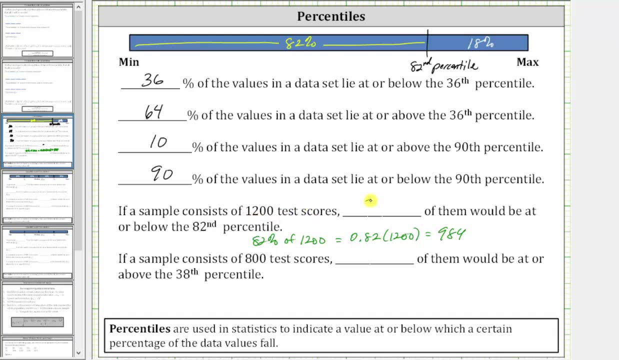 82% as a decimal is 0.82, giving us 0.82 times 1,200, which is 984.. Which means if a sample consists of 1,200 test scores, 984 of them would be at or below the 82nd percentile.